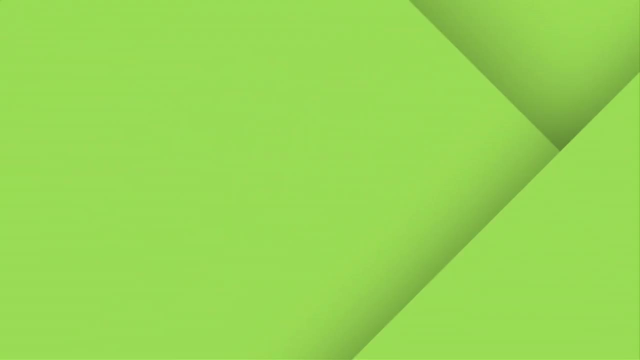 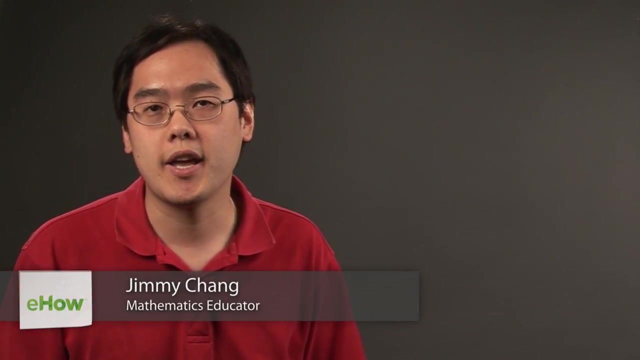 Hi, I'm Jimmy Chang, and we're here to talk about how to compute a number with a very high exponent. Now, when it comes to very high exponents, there comes a time when you may need a calculator to do it, but if you want to think about how to do it by hand, here's something to consider. 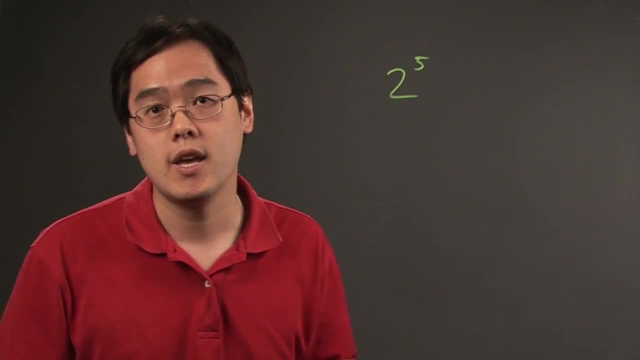 Suppose, for example, if you want to find out 2 to the 5th, Now, 2 to the 5th is like writing the number 2 multiplied by itself 5 times. Now one way you can break down a very high exponent is if you were to section it off. 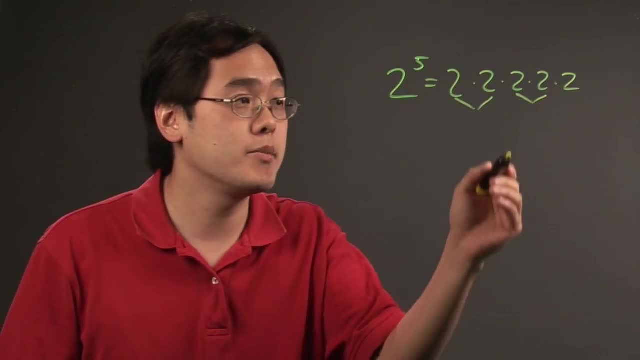 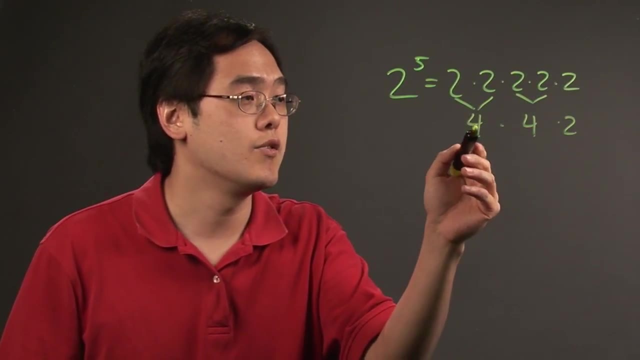 by breaking them off in pairs if possible. And for example, 2 times 2 is 4,, 2 times 2 is another 4, and then you're carrying that 2.. So 4 times 4 is 16, times 2 is going to be 32.. 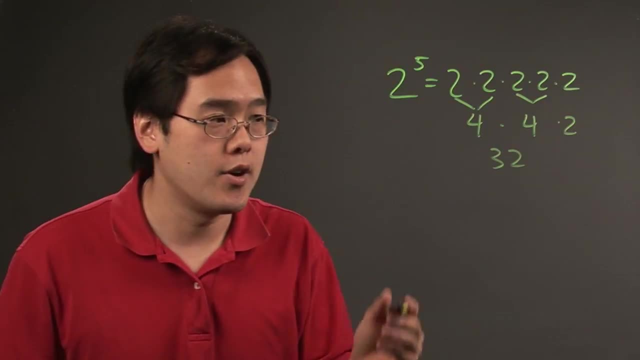 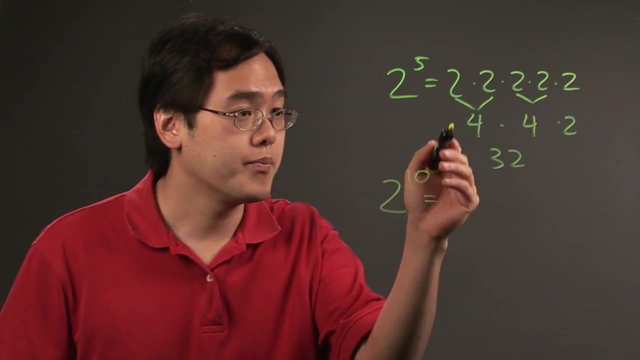 And 5 is not too high, but it's not very low either. Now, if you want to calculate a very high exponent like 2 to the 10th power, you can think of it as 2 multiplied by itself 10 times. 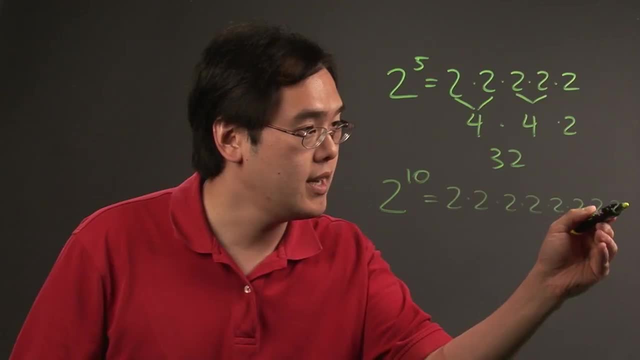 So 4,, 5,, 6,, 7,, 8,, 9, and 10.. Let's see 1,, 2,, 3,, 4,, 5,, 6,, 7,, 8,, 9,, 10.. 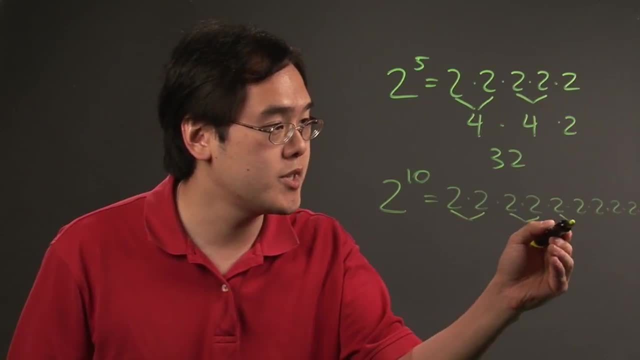 You can do the same kind of idea: Break them off into as many pairs as possible. So you have 4, 4,, 4,, 4, and 4.. Now what you can do is you can multiply all these numbers together. 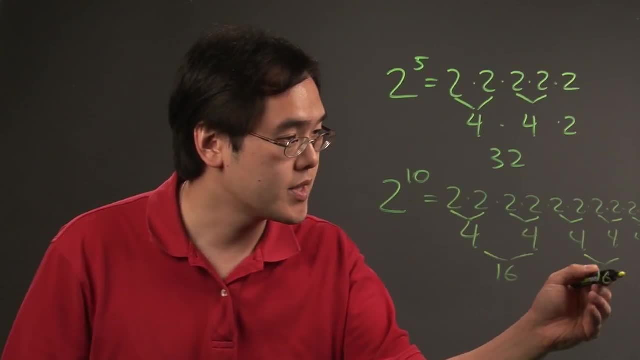 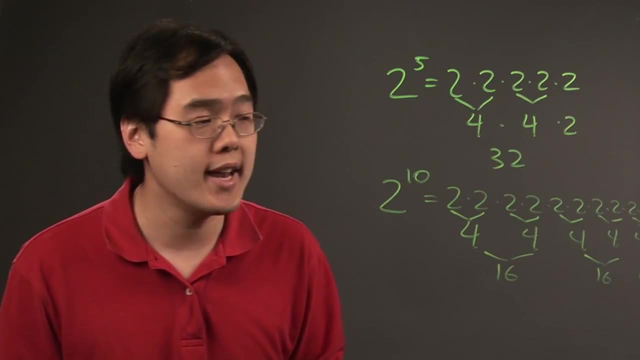 You could even do 16s if you like, 16 times 16.. 16 times 4.. And then just do the multiplication from there. But the understanding here is: the higher the exponent that you get, the more tedious it becomes. 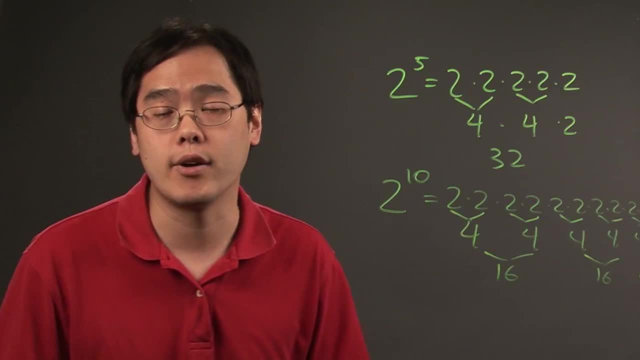 and that's where you might want to use a calculator for some of the heavy-duty calculations. So I'm Jimmy Chang and that's how to calculate a number with a very high exponent.